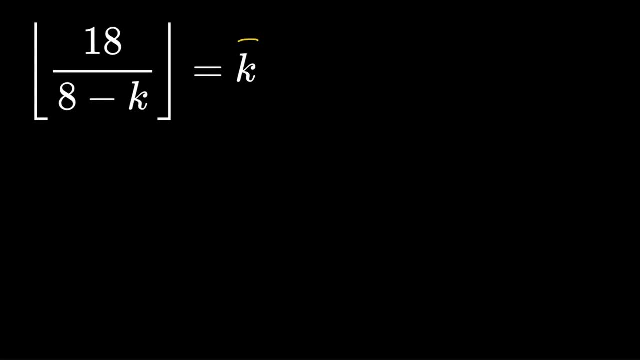 of application on the floor function. Well, k is the result of this floor function and because it is called the greatest integer function, k is going to be the greatest integer less than or equal to 18 divided by 8 minus k. So with that information alone, k would definitely be an. 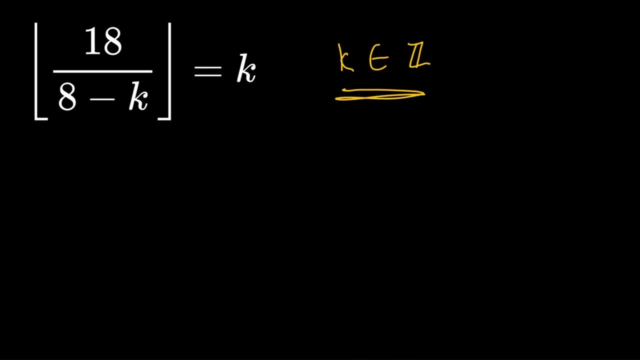 integer. right, That's going to be step one. Now, the other thing to note about the floor function is that, well, since we know that the floor, or the greatest integer, less than or equal to the 18 divided by 8 minus k, that's going to be greater than or equal to its floor, which is k. 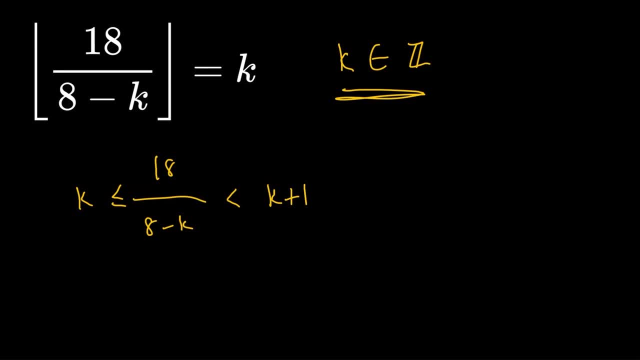 and it must be less than the next integer. So that's a very nice property actually. Whenever you have a floor, let's just say floor of a, let's just say we got this to be k. or, let me use a different level, let's just say it's m, then a would have to be between m and m. 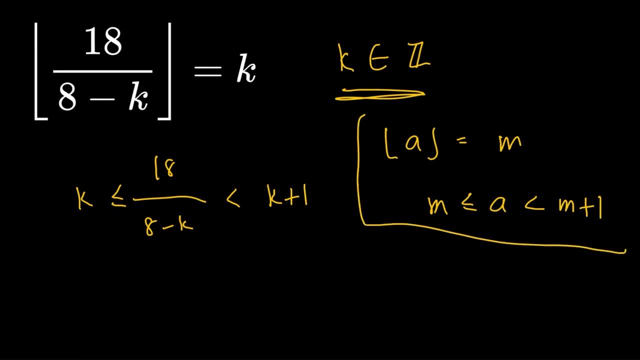 plus 1.. So it's going to be greater than or equal to m, but less than m plus 1.. So this is a nice thing that you could use for the floor functions, because it gives you a bound. So for questions that involve the floor function, there's going to be a lot of bounding. taking a look at the 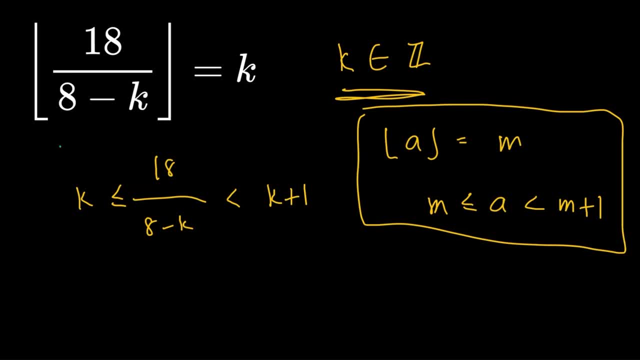 integers and something like that. Now we do have this inequality. I'm just going to focus on the left and the right one. I'm going to split them. The first one is going to be this: And all right, this is a rational inequality. So I'm just going to do the standard way on. 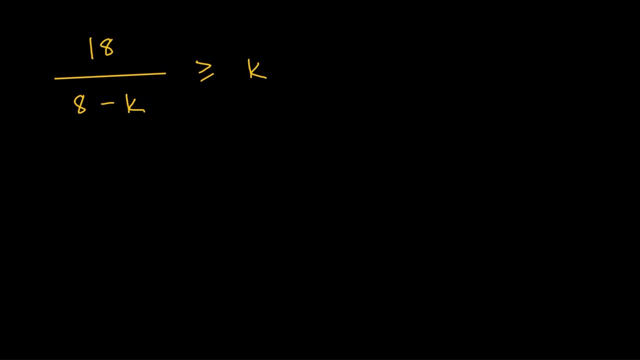 solving them. Here's another video on solving rational equations. Click this link and that's going to give you the other example on rational inequalities. Now I'm just going to move the k to the other side, So I'll have minus k times 8, minus k divided by. 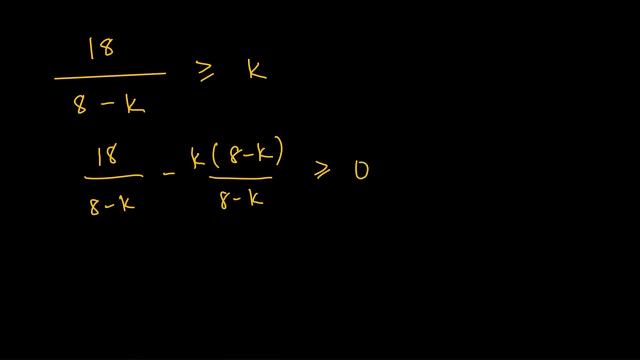 8 minus k, And this would be greater than or equal to 0.. And putting it into one fraction, I'll have 18 minus 8k plus k. squared divided by 8 minus k, That's going to be greater than or equal to 0.. Now there's one funny thing: actually The numerator. 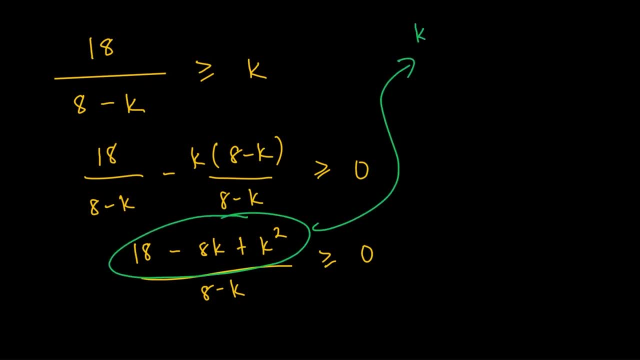 I can write this as k minus 4, squared plus 2.. So, in fact, well, this thing is always positive Because, well, it's 2 more than a perfect square, and k is a real number, So the numerator is always. 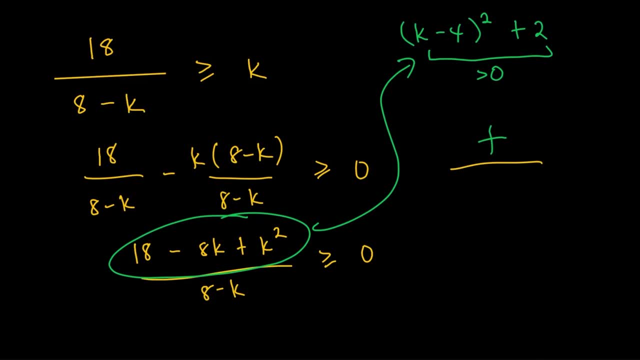 positive. So a positive number divided by 8 minus k, it's going to be greater than or equal to 0.. So well, it can't be 0 because the numerator is positive, But surely this 8 minus k that has to. 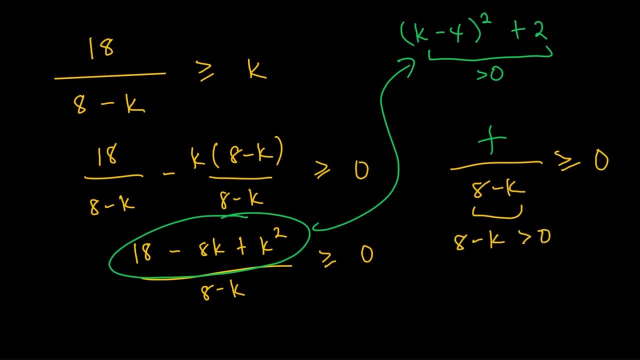 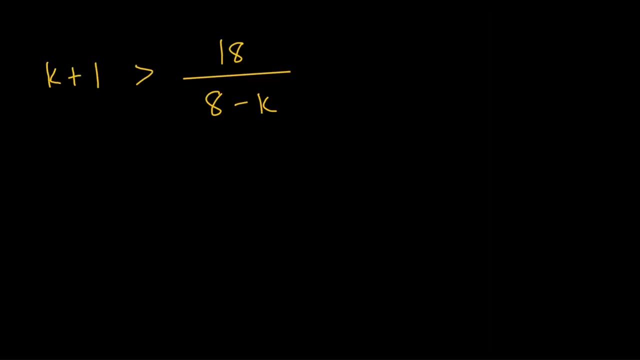 be positive as well. So 8 minus k must be greater than 0.. That's going to give us k to be less than 8.. That's going to be one bound for the question, which is pretty good, All right. Next, let's try to focus on the next part: k plus 1 being greater than 18 divided by 8. 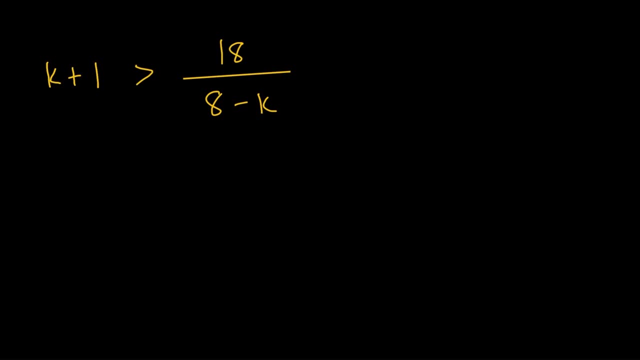 minus k. Same trick. Let's try to do the standard way. I'm going to put the k minus 1 to the other side, So we're going to have this one, And then I'm going to write the k plus 1 now as 8 minus k. 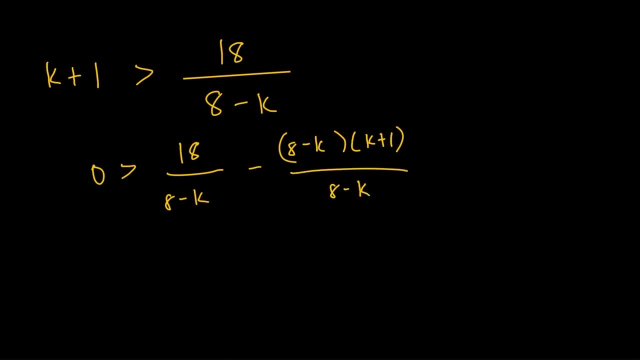 times k plus 1, divided by 8 minus k, With the goals of writing the expression in terms of this one fraction. So it's going to be 18 minus 8k minus 8 plus k, squared plus k. All right, And let me just simplify the numerator. So I'll have 0 to be greater than. 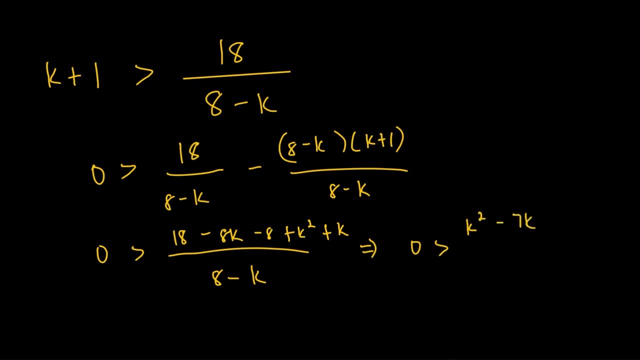 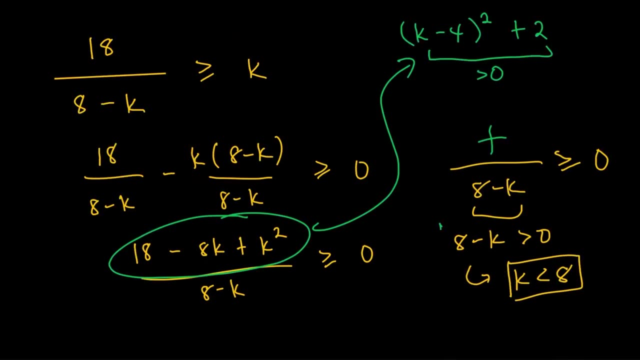 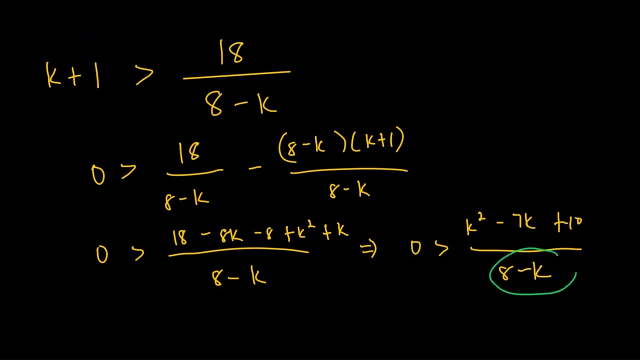 k squared minus 7k plus 10, divided by 8 minus k. Now take a look. We have 8 minus k to be greater than 0 from the first one. We could use this to our advantage. So 8 minus k is going to be positive. So if I multiply both sides by 8 minus k, 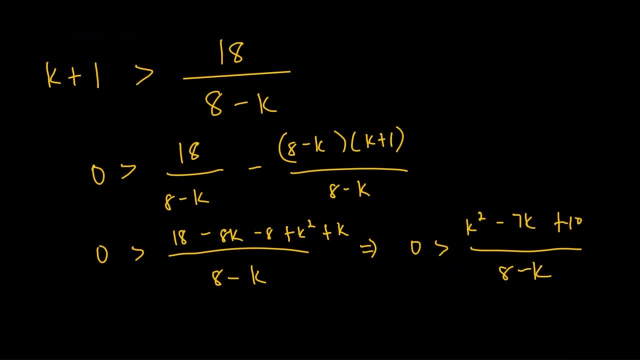 the inequality sign will not change the direction, So that's good. So I'm going to multiply both sides by 8 minus k. I'll have 0 being greater than k squared minus 7k plus 10.. And if I solve this inequality, I can factor the right-hand side. 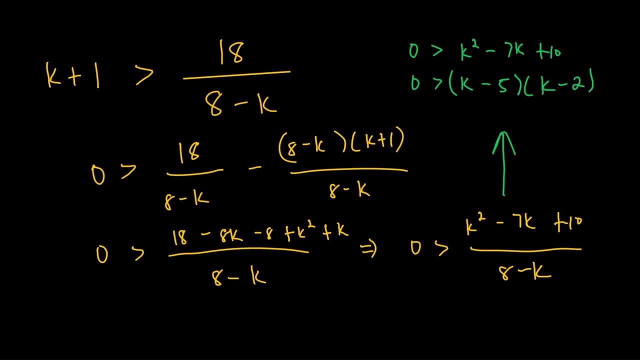 This one And I could solve the inequality. This is just a quadratic inequality. now I have two critical points: 2 and 5. So I know that the values of k must be between 2 and 5 exclusive. So just simply use the knowledge in quadratic inequalities over there Again, combining with 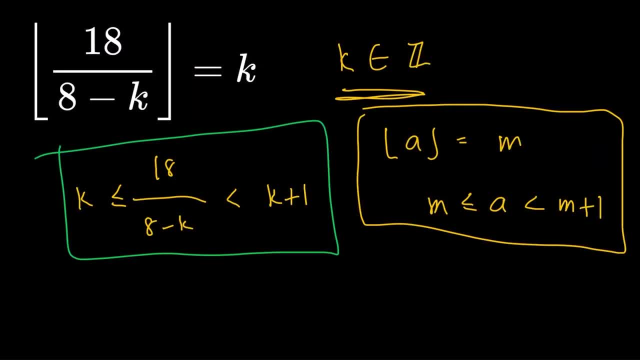 the fact that k is an integer. we just have to get integer values for k that's between 2 and 5, exclusive, And we could just kind of solve the inequality. So I know that the values of k must be between 2 and 5 exclusive And we could just kind of solve the inequality. So I know that the values